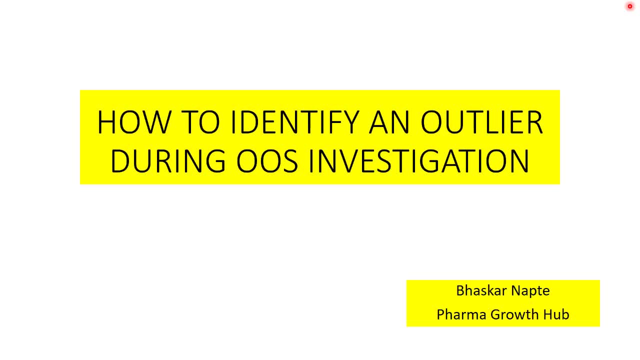 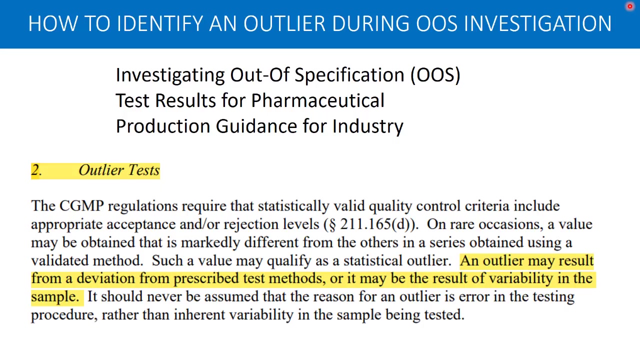 hello and welcome. so in today's video we will talk about how to identify an outlier during out of specification investigation. see, this is one of the challenge I often seen people face while investigating an OS. so if you look at the US FDA guideline on to the investigation of out of specification, 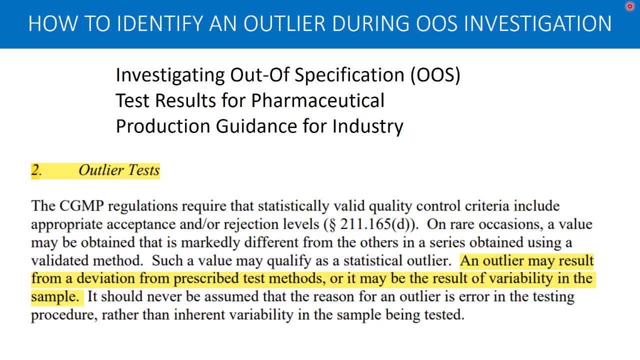 or even the guidelines given by the EMA, you will find that both of them. both of them mention of the outlier test. so regulators recognize that the analyst may come across outlier test result and that has to be investigated properly, based on to the statistical evaluation. now, when they say statistical, 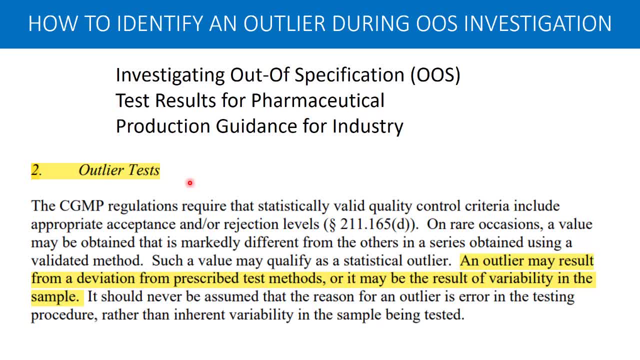 evaluation. the details of how one can reach to a conclusion whether the given measurement is really an outlier or not is not well explained into the guideline. so that is the purpose of making this video: so that you all can get an understanding how one can identify an outlier during. 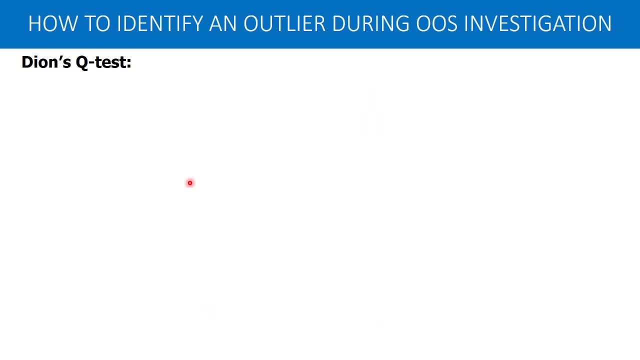 out of specification investigation. so so this is the test that is called as the Dianst Q test, and Dianst Q test will help us to understand an outlier within the given number of measurement. so I will walk you through very step by step, slowly, so that you can understand identification of an outlier. 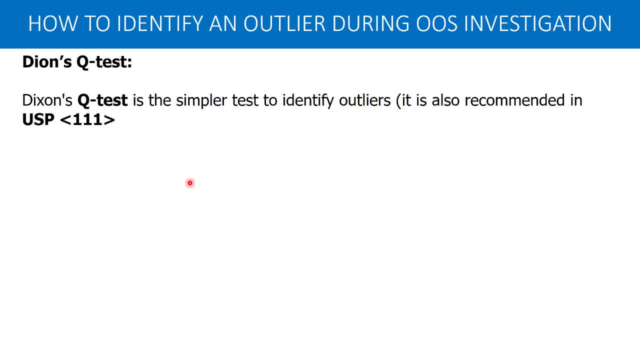 during an OS investigation. So it is not something that there is no at all a guidance provided about understanding an outlayer, but there is a USP General, Chapter 111, where you will find that the Diane's Q test is mentioned in identifying the outlayer test result. 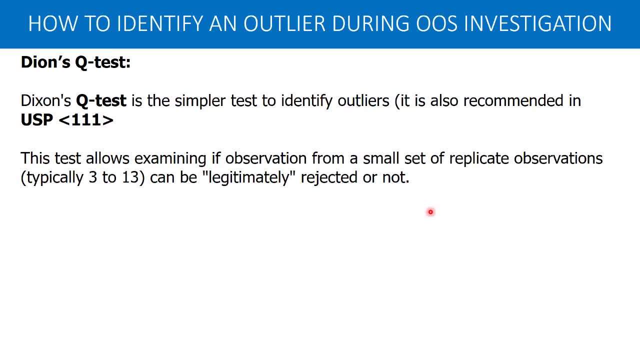 So this test allows examining if observation from a small set of replicate observations, typically in between 3 to 13, can be legitimately rejected or not. Rejected means what? If it founds to be an outlayer, then you can certainly reject that observation or the measurement. 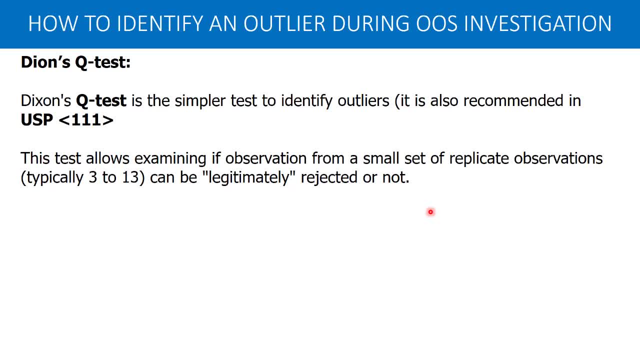 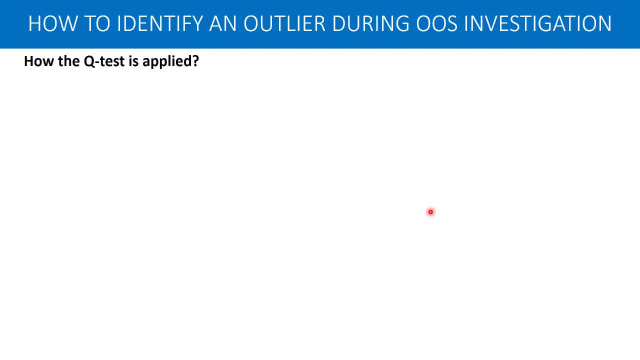 And this particular test is much applicable, reliable, typically for the number of observation between 3 to 13.. But then the question is how this Q test is really applicable To identify an outlayer. let us understand step by step. Number one, the n values comprising the set of observation under examination are arranged: 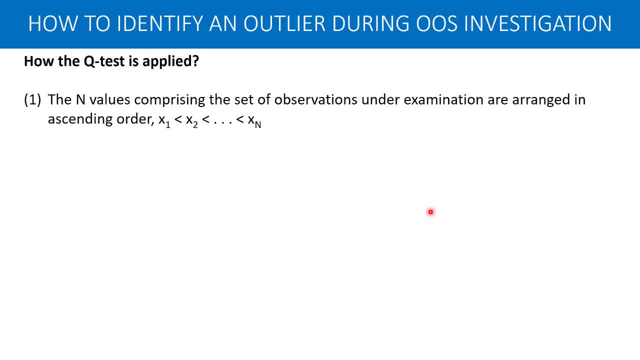 in ascending order. So, for example, you are conducting an assay and as a part of your measurement you're supposed to measure sample in triplicate. So you need to arrange These assay values in ascending order. means what In the increasing order. 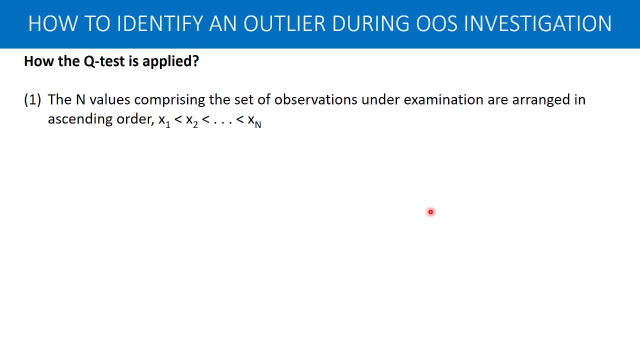 So the lowest assay value, let us say 99%, then the next value, let us say 100%, and then the highest value, let us say 101%. So this is called as the arranging the values in the ascending order. So you need to first arrange all your measurements in the ascending order. 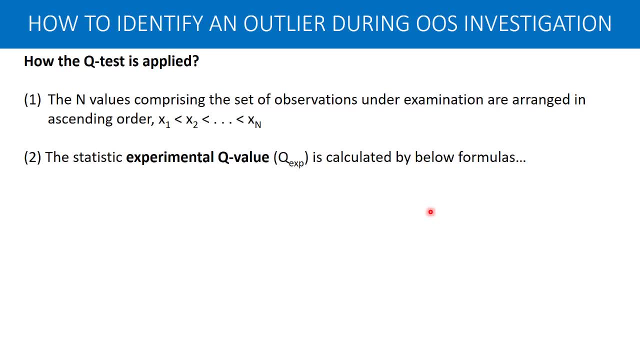 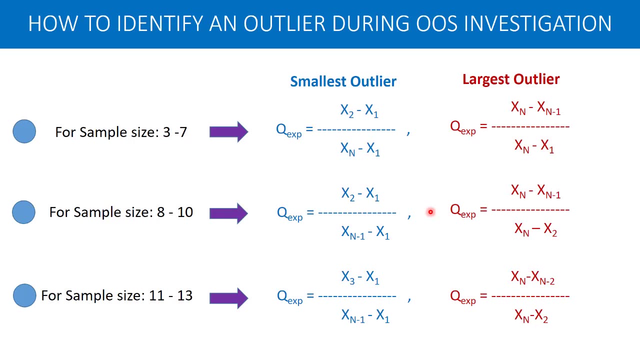 So once you make the arrangement, Then the second important step is the statistic experimental Q value. that is, Q experiment or QXP is calculated by below formulas. So in the next slide I will explain you the calculation of the Q experiment or Q experimental. 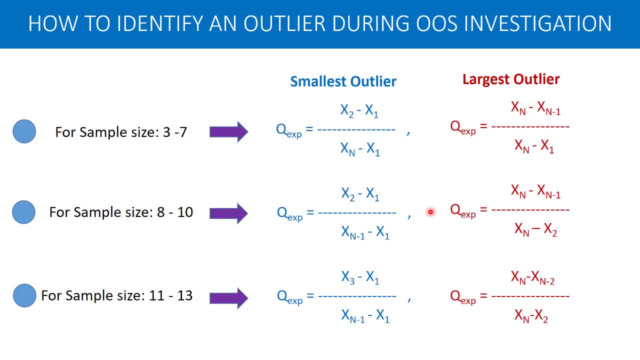 value for the given set of measurement. So if the sample size is in between three to seven, that means your measurements. if they are three or seven, then you have to calculate the Q experiment with this calculation formula, That is, X2 minus X1 divided by Xn minus X1, is going to give you the smallest outlay. 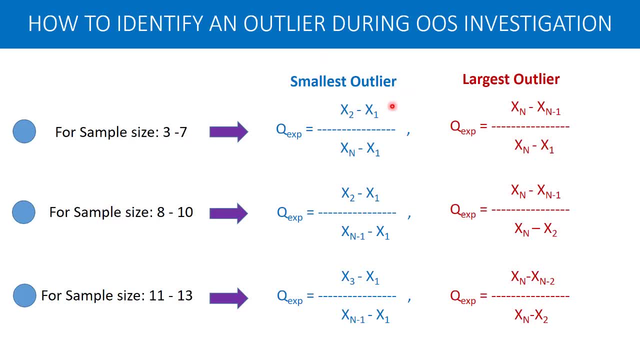 The smallest means what See in observation. let us say you have n number of observation, So there are possibility that either your first observation, the smallest observation, is going to be an outlay, or maybe the highest observation is going to be an outlay. 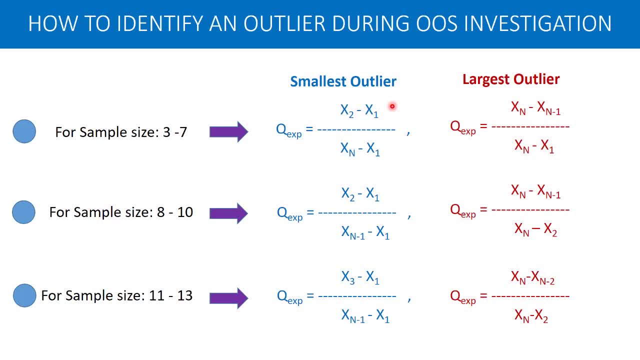 In between observation. they will not be outlay. Outlay means what? Observation lying on the border, Border means what They can be, either smaller value or the higher value. So there are two calculation formulas. The first calculation formula that I have just explained you for understanding the smallest. 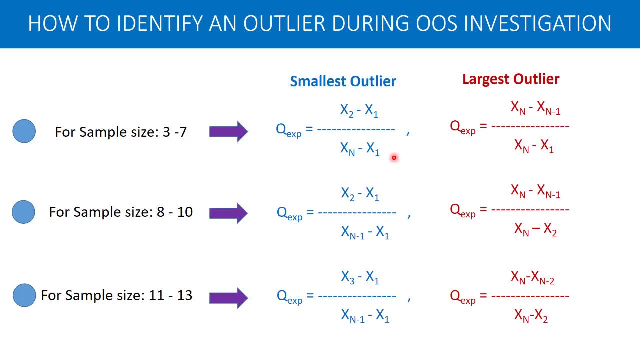 possible outlay. So if your sample set Or measurement contain the smallest outlet, then this particular calculation formula is going to give that. Similarly, the largest outlay can be calculated with this calculation formula: Xn minus Xn minus one divided by Xn minus X1.. 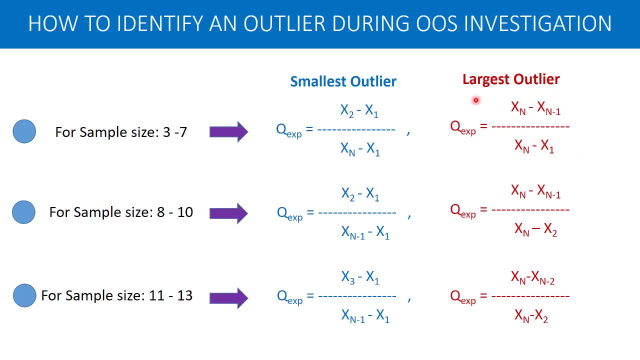 You can note down the calculation formulas or you can take the screenshot so that we will have this calculation formula with you. Now, this is for the sample size of between three to seven, But in case If your sample size is greater than seven, can the same calculation formula applies. 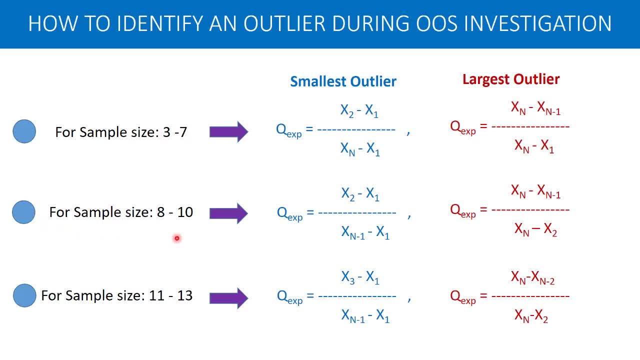 No. Then there is a calculation formula given for the sample size for eight to ten, And you can note down the smallest outlay calculation formula, Similarly, the largest outlay calculation formula. In case if your sample size is greater than ten, Again you have to apply a different calculation formula, which is given in the last. now. 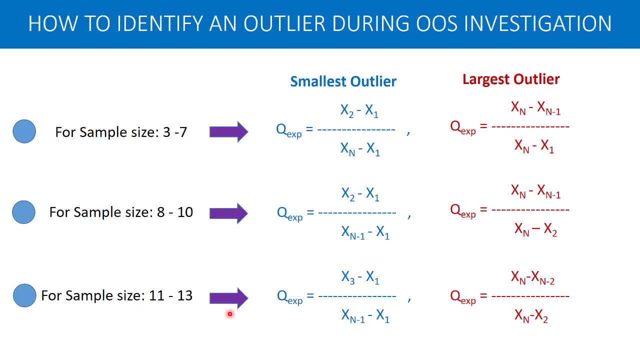 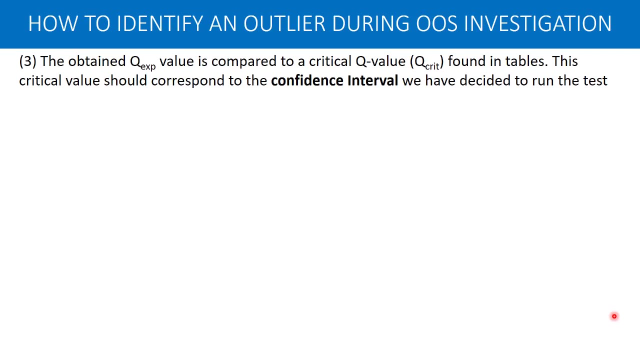 Though, If the sample size is between eleven to thirteen, then you can apply these two calculation formulas to calculate the smallest outlay as well as the largest outlay. I hope you are clear until this particular step. Then the next step is what? 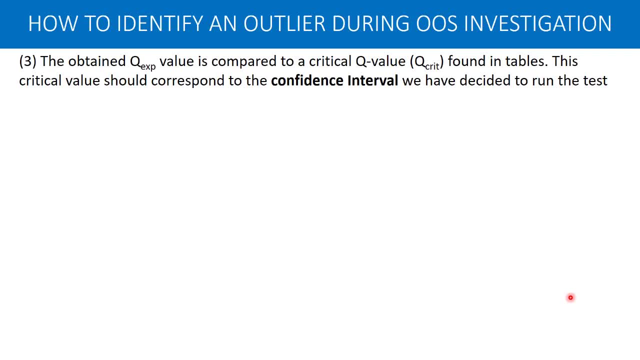 The obtained Q experimental value. Right, You understand the calculation formulas now and by using those calculation formulas now you are going to calculate the Q experimental values. So once you obtain the Q experimental value, then it is compared to a critical Q value, which is called as the Q critical found in the table. 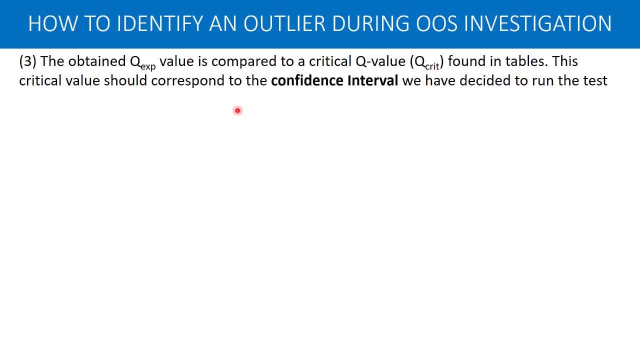 So I will let you know what is the Q critical values. And this critical value should correspond to the confidence interval. we have decided to run the test. See, each measurement is always done with a certain degree of confidence interval. You must have heard about the confidence interval. 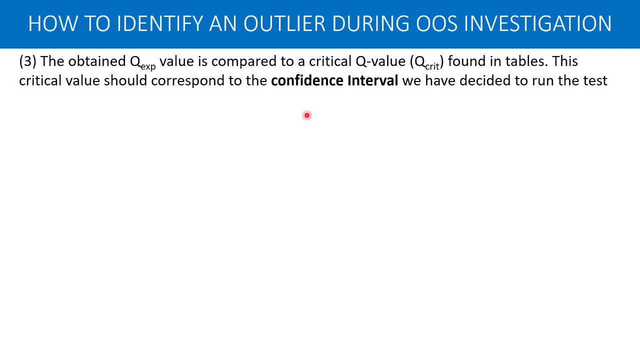 You must have heard about the confidence interval, So it is its result which reflects, which leads to the confidence interval. Does that include people who speak 95% confidence or 99% confidence? So this particular value is reported with a 95% confidence interval value. 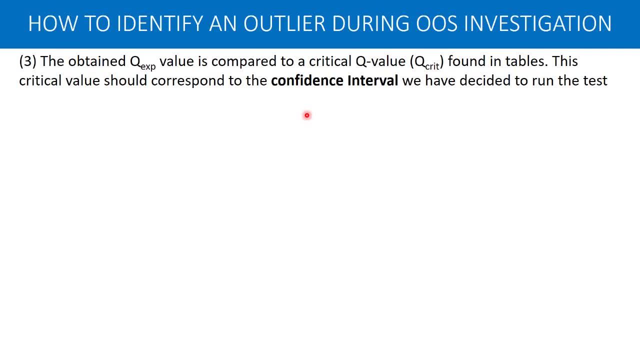 This is the value, as familia mentioned in the previous chart, Always rolling your confidence interval with the Q critical kalau depends on the confidence interval. That means if your confidence interval is different from when the external culture is connecting and the external frequency is not so fleshed out, then you cannot do much. 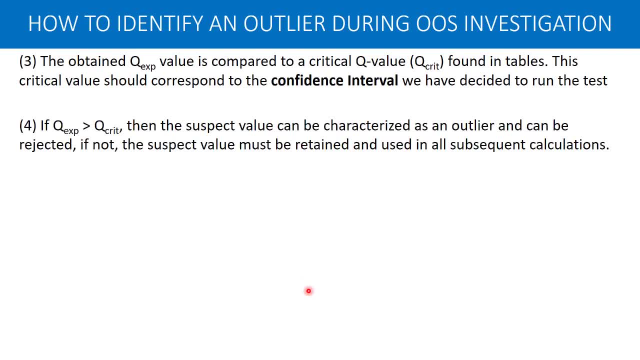 have the different q critical value. so let me bring the q critical value very soon. but before that, once you have the q critical value, then if q experimental value is greater than q critical value, then the suspect value can be characterized as an outlier and can be rejected. if not, the 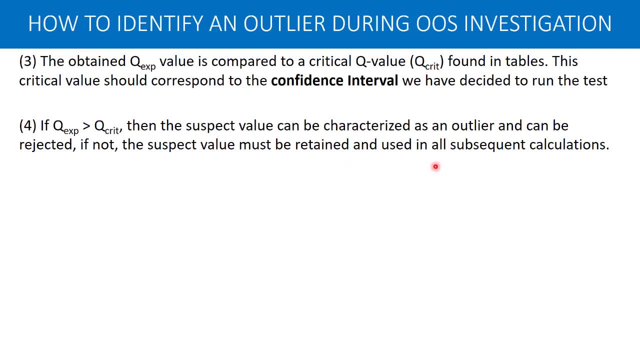 suspect value must be retained and used as i must be used in all subsequent calculation. that indicates that if the q experimental value, if it is greater than the q critical value, then you can reject that value, saying that it is an outlier. but if the q experimental value is, 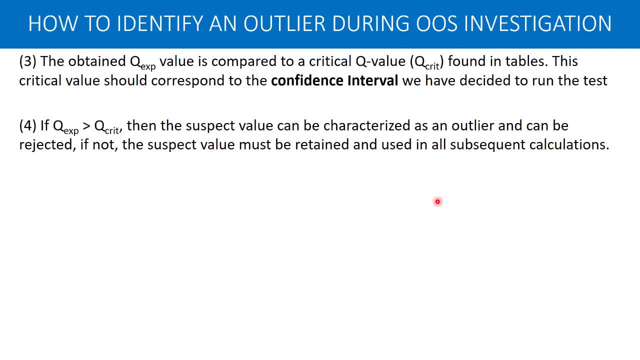 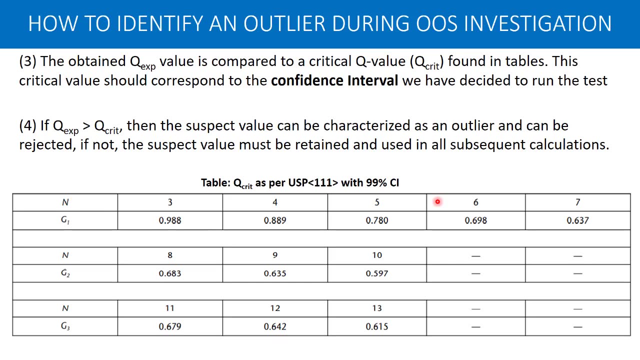 less than k critical value, then you cannot reject that value because that stands not an outlier and you must use that value for subsequent calculation. i hope you understand on this very important point. and then again, this is the the table which mentioned the q critical values and you will find this q critical values given in the usb general, chapter 111, and this: 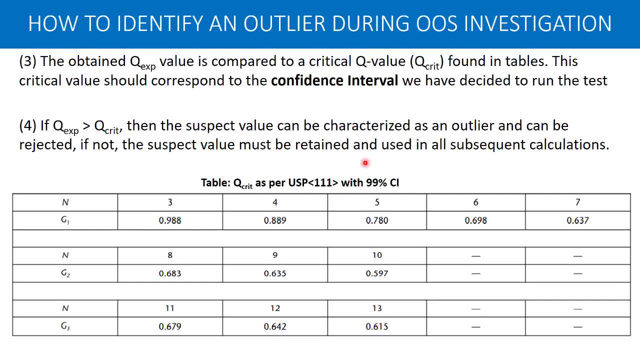 q critical value belongs to the 99 percent confidence interval. so if you are going to calculate the q critical value, then you must use that value for subsequent calculation. if you are going to define the outliers corresponding to the 90 percent confidence interval, then this particular values won't apply. or even if you consider to calculate the critical values, 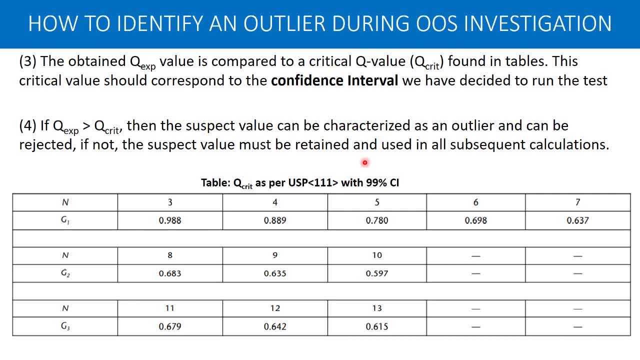 with respect to 95 percent confidence interval, then this table will not apply. so please remember this point: that this particular q critical values are within 99 percent confidence interval. so you can find that these are the confidence interval values. so g1, g2, g3, they are nothing but the the q critical values with respect to the number of measurement for 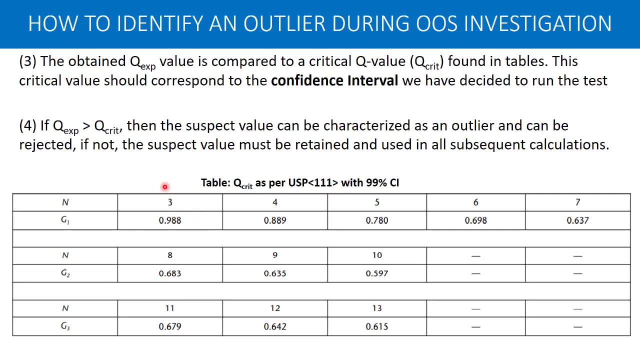 example, if the number of measurements are three, then what is your q critical value? 0.988, understand. if your number of measurements are four, then what is the q critical value? it is point eight, eight, nine, similar. Similarly, what is the Q critical value in case of your number of measurements are 30,? 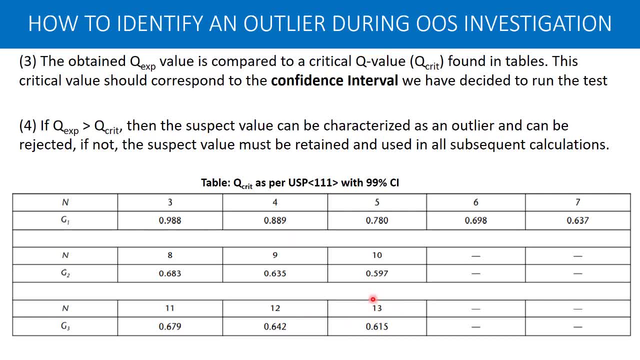 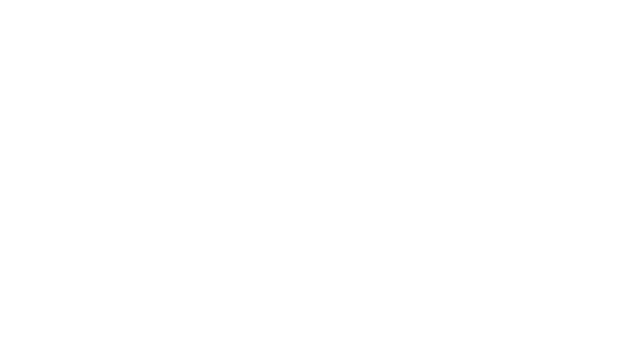 you can see over here right, The number of measurements are 30, your Q critical value is 0.615.. So I hope you are clear on this very important information. So, before we move on to the example, I would like to your kind attention that you know. 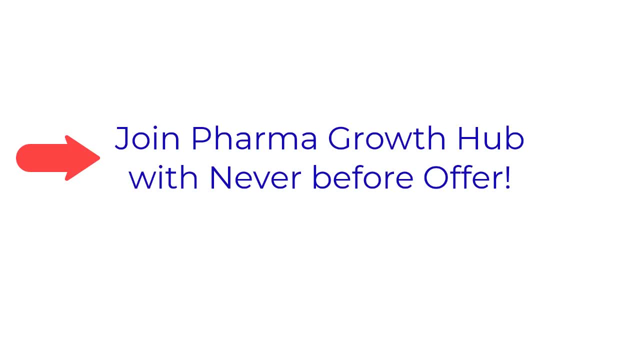 there are more than 1000 pharma professionals. You have chosen Pharma Growth Hub as their career acceleration partner. I am the founder of Pharma Growth Hub And I am on the mission to help pharma professional to boost their career growth by providing absolute clarity on various topics, by creating an ecosystem where professionals can network. 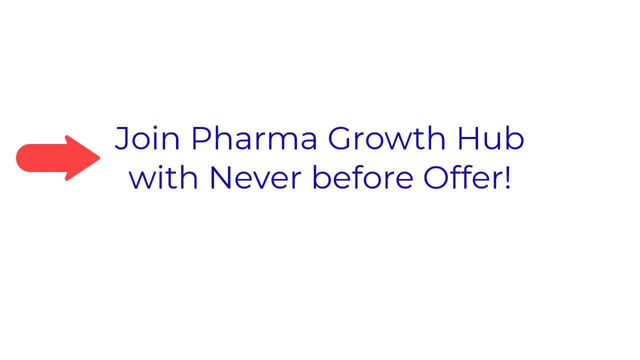 and help each other to identify new opportunities. So, in case if you are finding a stagnancy into your career growth, not able to understand how to identify the new opportunities, new job opportunities, there is a way to go. so there is an opportunity to become a lifetime. 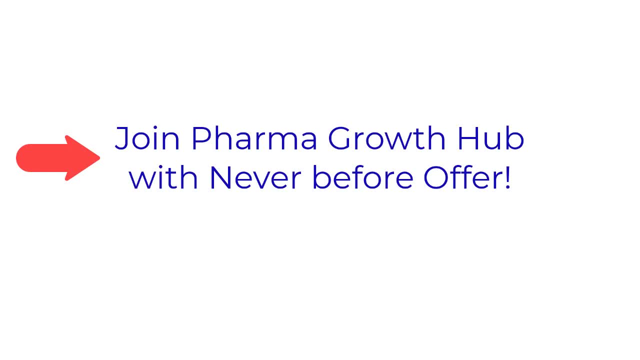 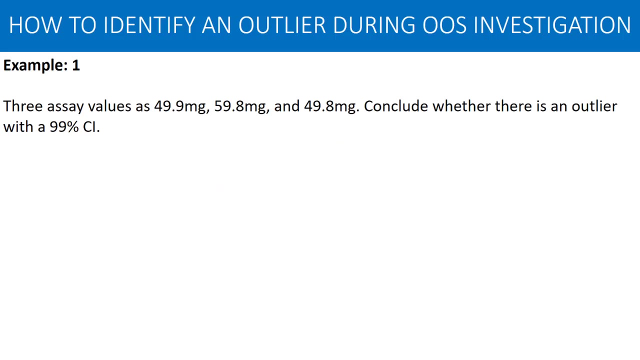 member of the pharma growth hub with never before offer. if you are interested, please check the details given in the description below and join pharma growth hub today. thank you so much. so let us understand the calculation of, or identification of, an outlier with a very simple example and you. 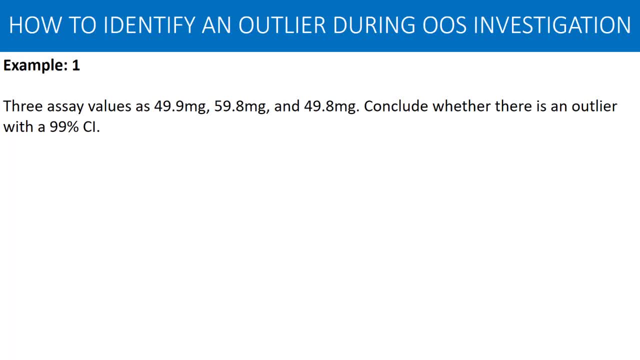 can see example onto your board. so let us say you have three different assay values, with the 49.9 mg first observation, 59.8 mg second observation and 49.8 mg as the third observation. so you want to understand whether there is any outlier value within these three different measurement and you 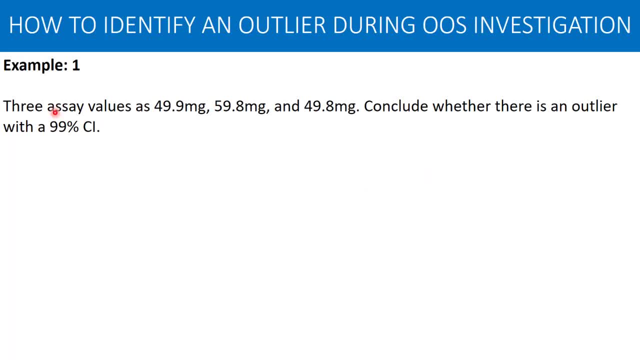 are going to consider this outlier measurement with the 99 confidence interval value. so please remember there is a. you can see example onto your board. so let us say you have three different assay values with the great use connection of this confidence interval. what is the step number one? arrange this values. 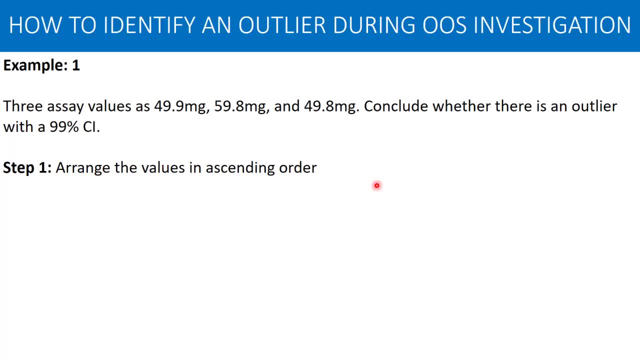 into an ascending order, means in the increasing order. so i have arranged all them into the increasing order. and then again there is a step number two that determine the q experimental value. so by using the now, as this number of measurement are three, i hope you remember i have shown you. 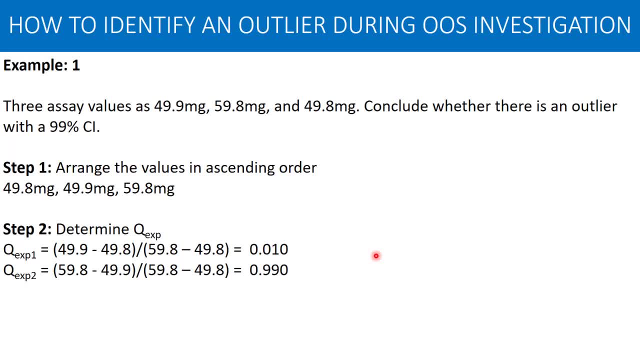 the calculation formulas for q critical values. so by using that calculation formula i have you. i have calculated the q experimental, q experimental- for the smallest value, right, that is the q experimental one. i just notified that with the different notification so that i can differentiate what is q experimental one and q experimental two. 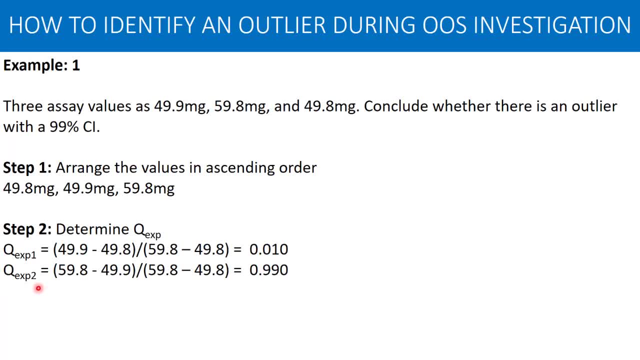 so q experimental two is the q experimental value for the highest, uh the outlier possible value. so i understand that now the q experimental one is 0.010 and the q experimental 2 is 0.990 in the step number three. now i need to compare the q experimental value with the q. 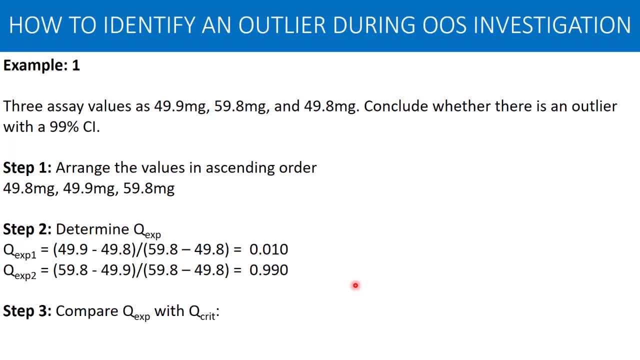 critical values and what is the source of the q critical value? do you remember the table? same table. i will consider, and let us say that you know, the q critical values with the three measurements, with 99 confidence interval: is: how much is 0.988? is how much 0.988? see in the next step now what i